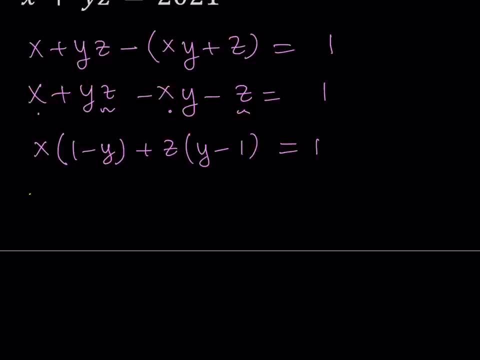 go ahead and do this. I want to put a negative sign here with the x, so that I can make this y minus one, And the second one is going to stay the same. Then now, since we have y minus one as a common factor, let's just go ahead and write it as z minus x. I just interchange those two terms. 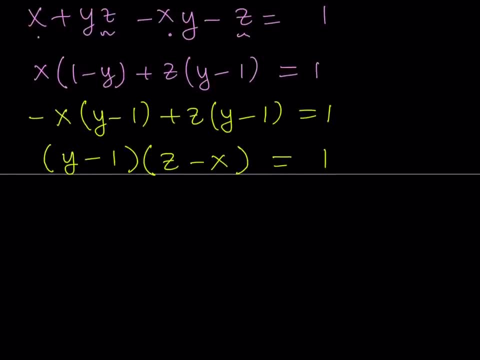 and this equals one. Now, this is significant because one can only be factored into one times one and negative one times negative one. So we're looking at two cases. Let's take a look at case number one. So case number one is: if y minus one is equal, 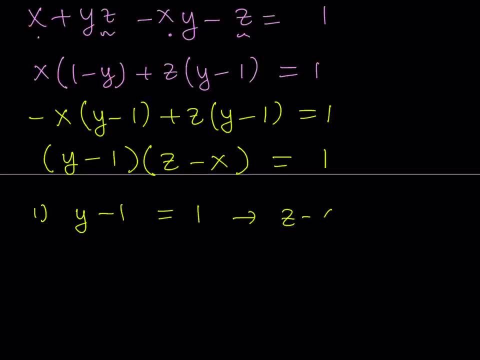 to one. That also implies that z minus x equals one. So one times one equals one. Great. So y equals two. from here Now, obviously, I would like to find x and z as well, but I only got one equation. We can go to the original ones. 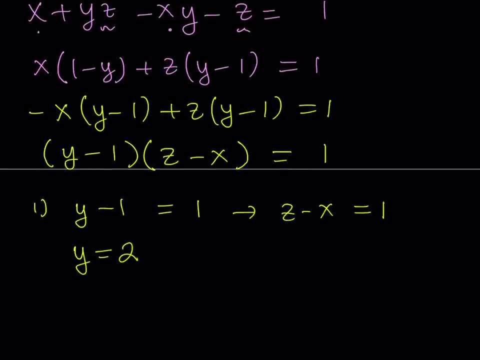 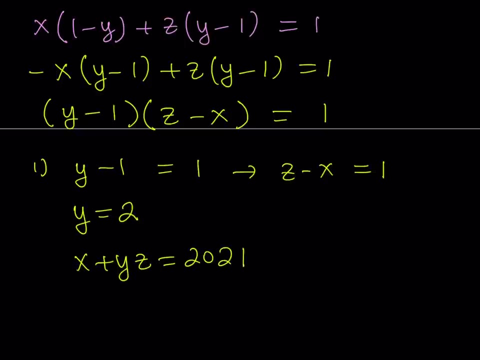 And see if we can replace y with two, And I'd like to use the second equation. The second equation is: x plus yz is equal to 2021.. If you replace y with two here you get x plus 2z or not 2z. well it. 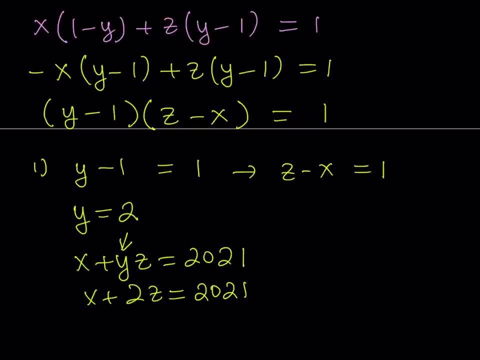 didn't fit, equals 2021. And let's go ahead and solve this system by elimination. So I'd like to add these two equations: x cancels out. We get x plus 2z. So we get x plus 2z. So we get x plus 2z. 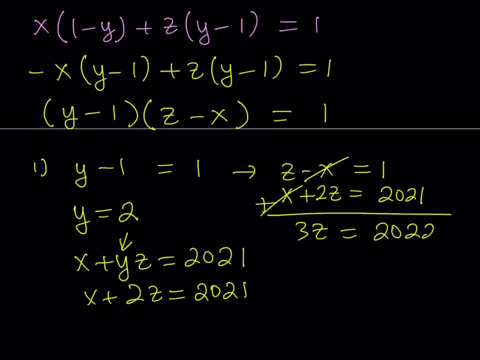 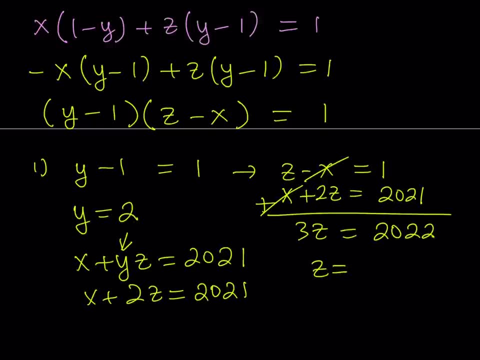 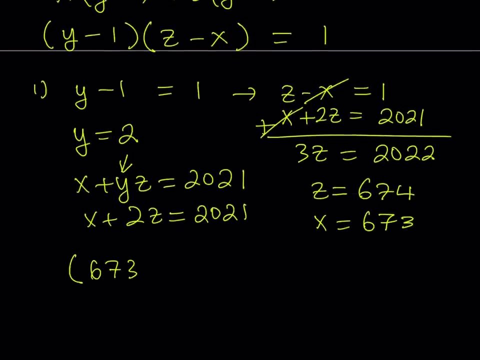 Divide both sides by three, You get z equals 674.. Since z and x differ by one, x is smaller, x is going to be 673.. So this gives us the ordered pair 673. comma 2 comma: 674.. Okay, Let's look at. 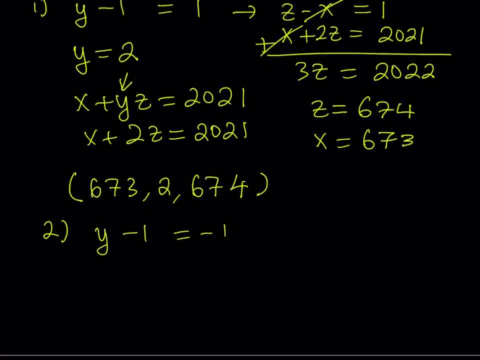 the second case: If y minus 1 is equal to 1, then y minus 1 is equal to 1.. So if y minus 1 is equal to 1, then y minus 1 is equal to negative 1. This implies that y is equal to 0, which is kind of.